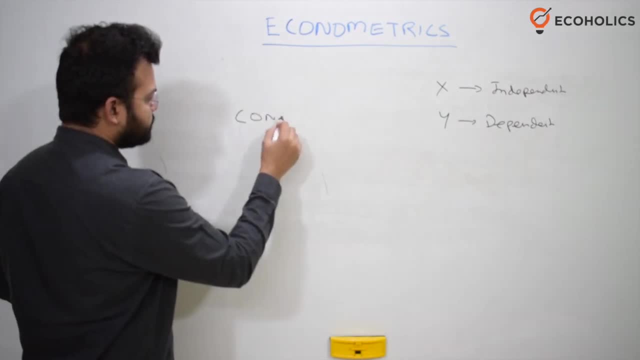 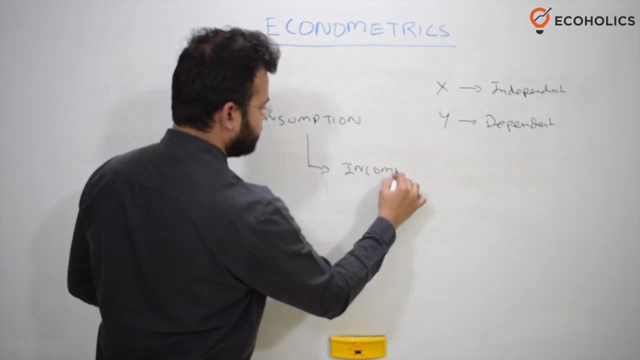 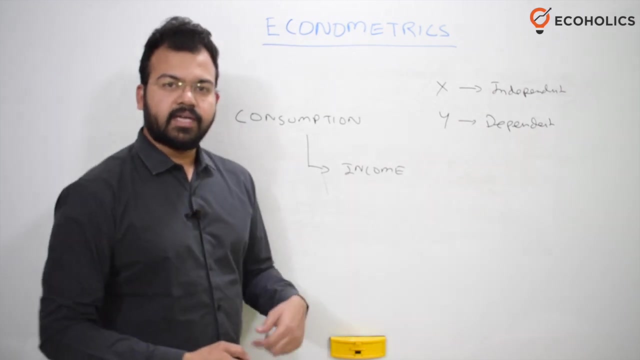 Like. suppose, for example, your consumption depends on income. This is very simple. So whatever you are consuming, it depends on your income. Suppose you are eating chapati. you are eating bread, you are eating non-vegetarian dishes, you are eating certain luxury food. 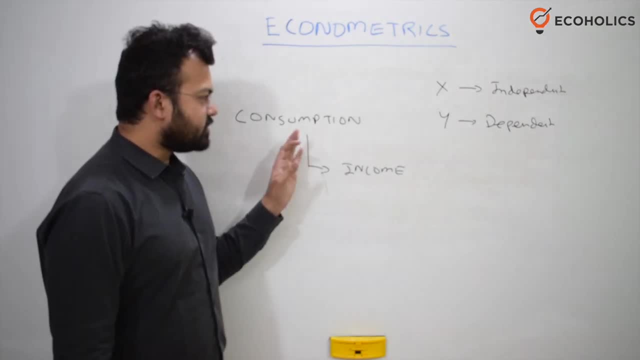 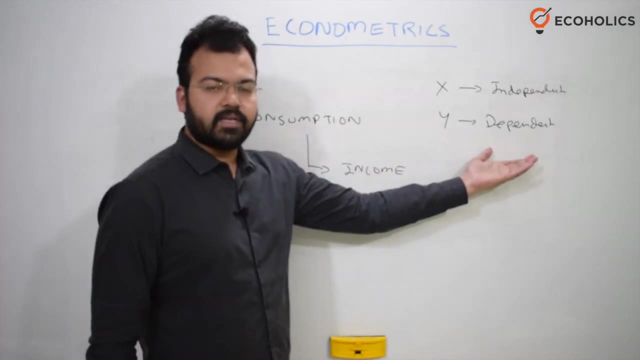 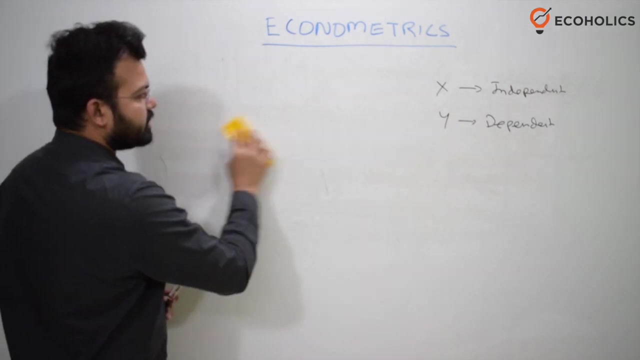 It depends on the income. So that is the basic notion, that your consumption is dependent on the income. Here we can say that your consumption is the dependent variable. your independent variable is the income. So let's see in the form of the equation in the simple linear regression model, where 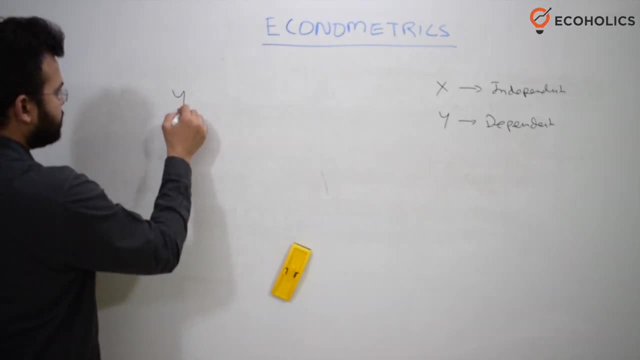 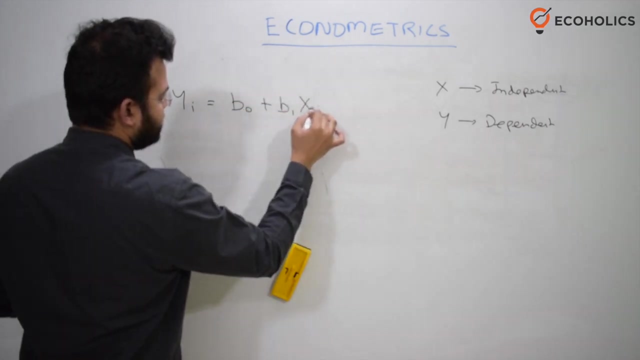 we can decide this. Suppose the equation is: Y is equal to B0 plus B1 X. So what we can do here is: we can write this equation, So we can write this equation here. We can write this equation here. We can write this equation here. 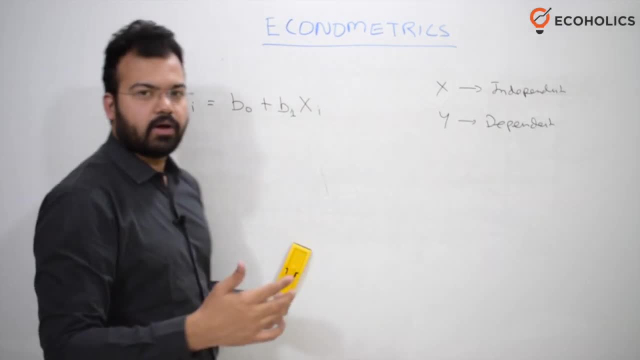 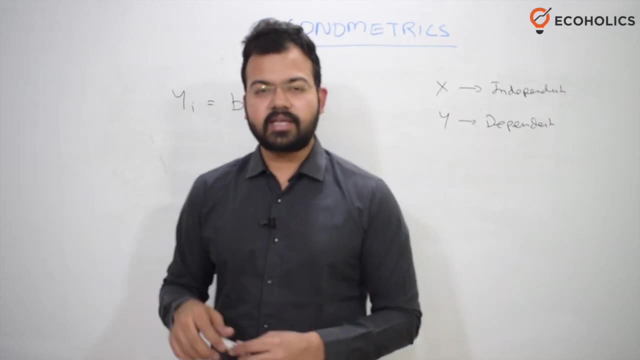 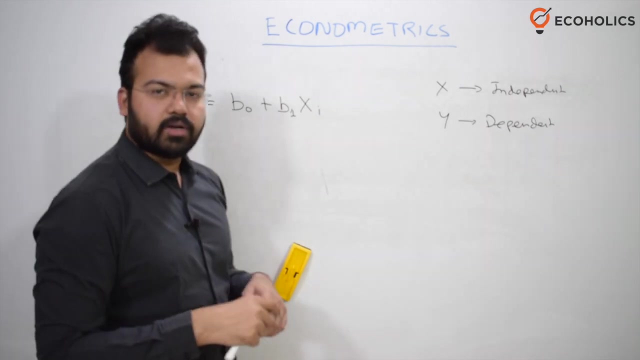 So here we can say: this Yi is obviously your consumption, and here this Xi is your independent variable, That is here, in our case, is the income. So here we can say that this Y is dependent on the income level or the consumption dependent on the income level. 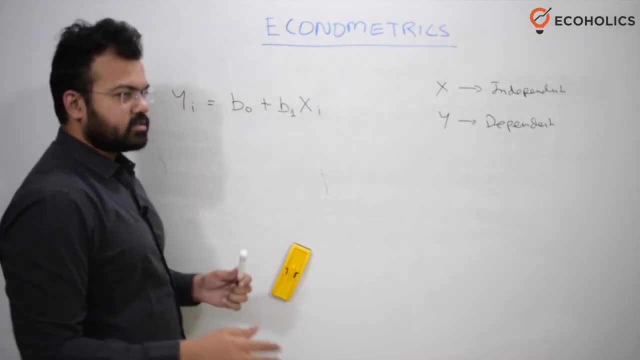 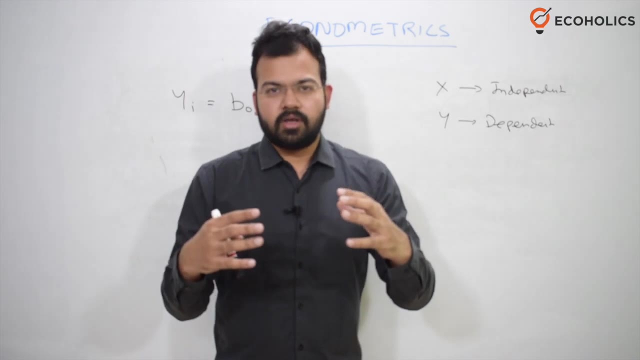 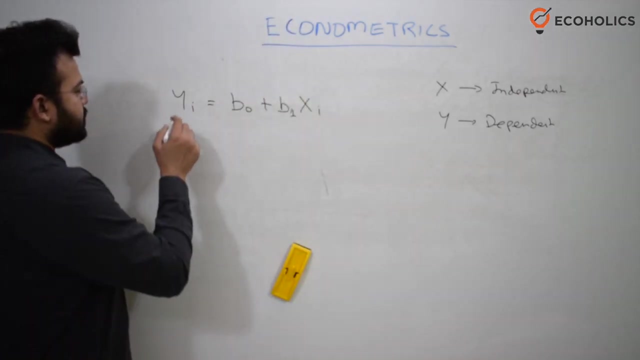 So as your income goes up, your consumption will also go up. This is a basic theory in economics: As your income goes up, your consumption will also go up, But obviously not in the same proportion Or not on the same increment. So here the important thing: we need to understand that this is the dependent variable and this 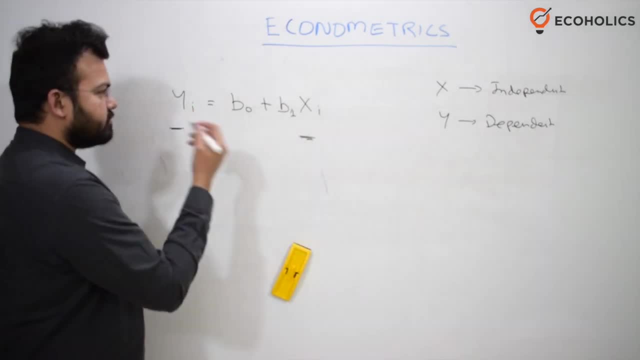 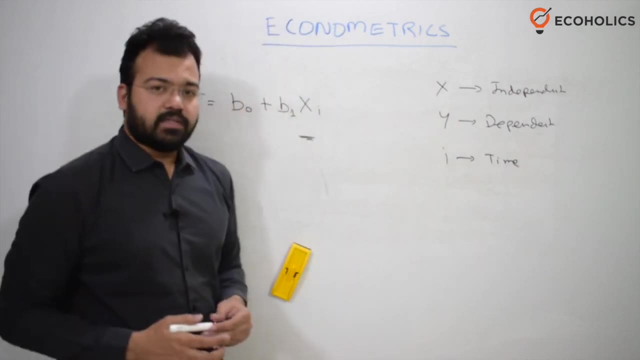 is the independent variable. Now the question arises: what's the meaning of this? I- Here we can say I is certain time period. So here it may be the particular year of time series data, or it may be a particular unit of any cross-sectional data. 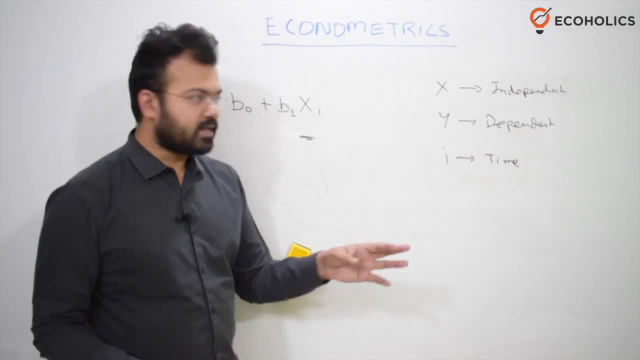 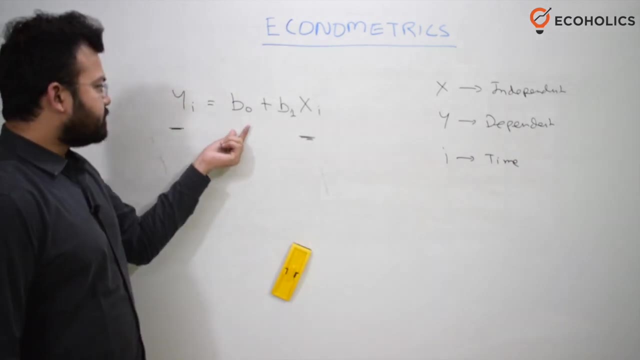 So there are different types of data, like time series data, cross-sectional data, time series data, panel data, etc. So here this I small. i refers to certain time period. Now, what is B0 and B1?? Here B0, we can say, is the autonomous consumption. 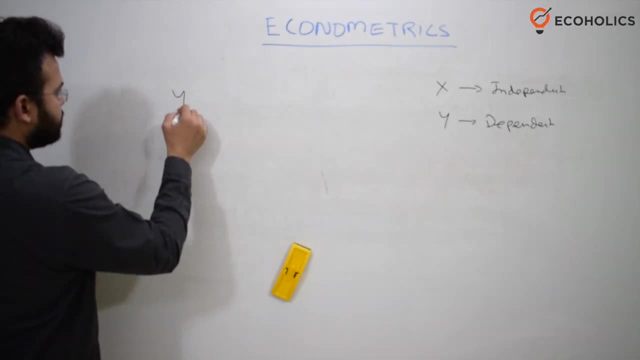 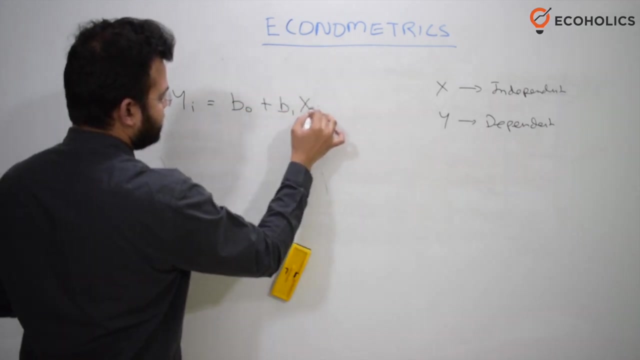 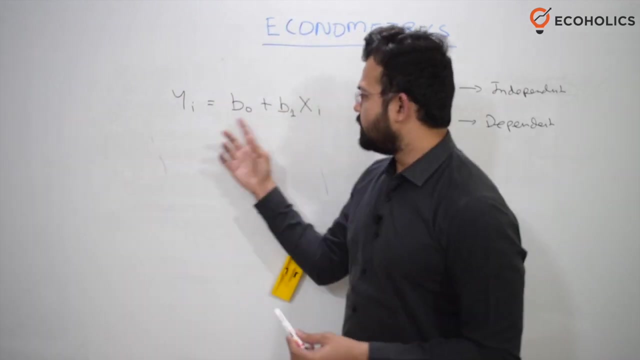 we can decide this. Suppose the equation is: Y is equal to B0 plus B1 X. So what we can do is we can use this equation. We can use this equation to calculate the consumption. So here we can say this: Yi is obviously your consumption and here this: 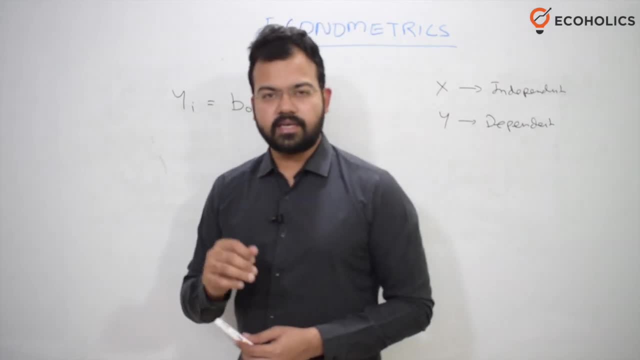 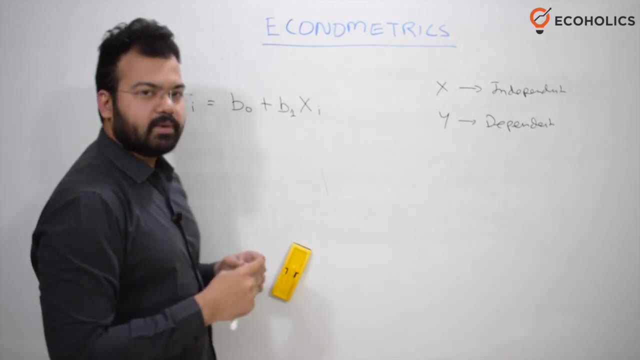 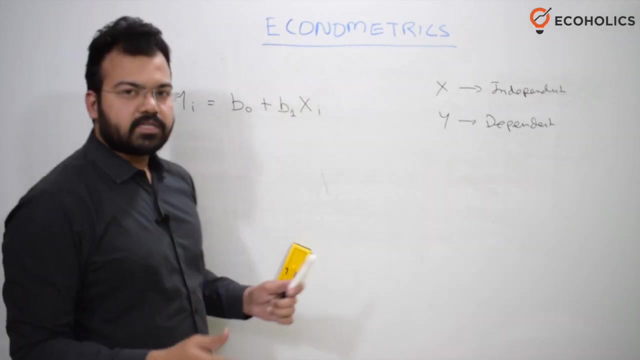 Xi is your independent variable. That is here in our case, is the income. So here we can say that this Y is dependent on the income level or the consumption dependent on the income level. So as your income goes up, your consumption will also go up. This is a basic. 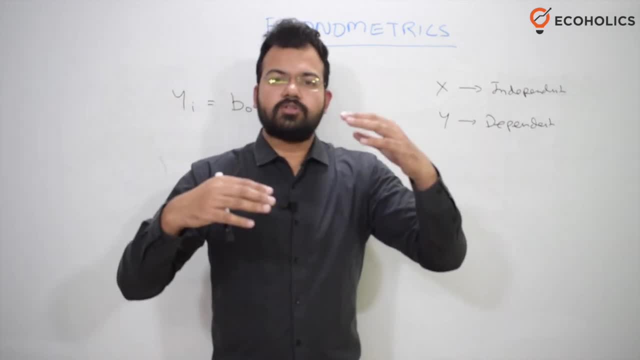 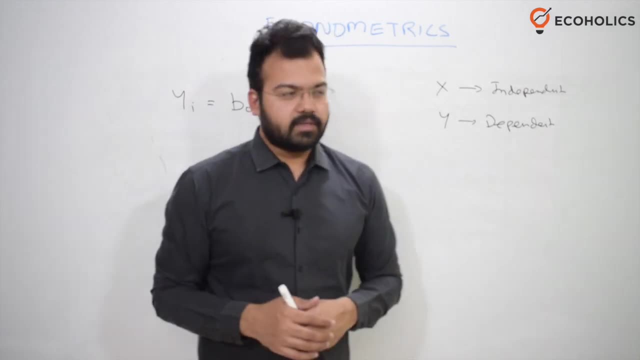 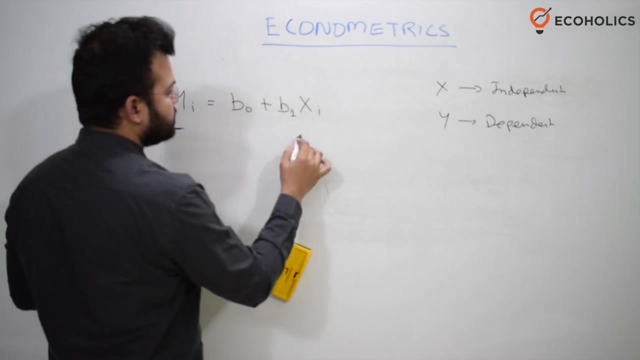 theory in economics, As your income goes up, your consumption will also go up, but obviously not in the same proportion or not on the same increment. So here the important thing: we need to understand that this is the dependent variable and this is the independent variable. 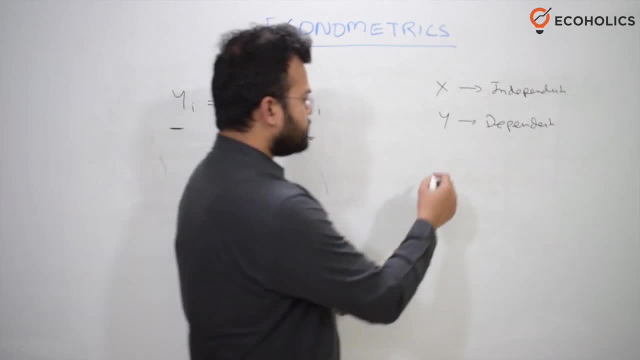 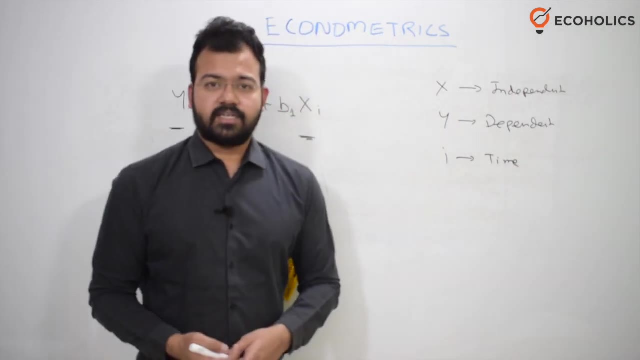 Now the question arises: what is the meaning of this Yi? Here we can say: Yi is certain time period, So here it may be the particular year of time series data, or it may be a particular unit of any cross-sectional data. So there are different types of data, like time series. 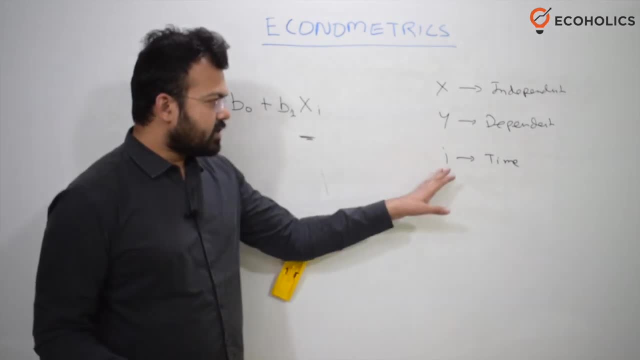 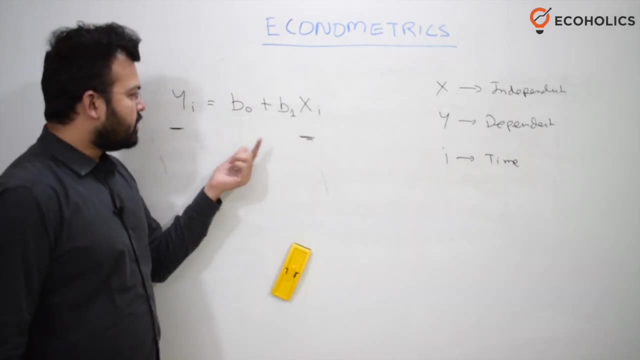 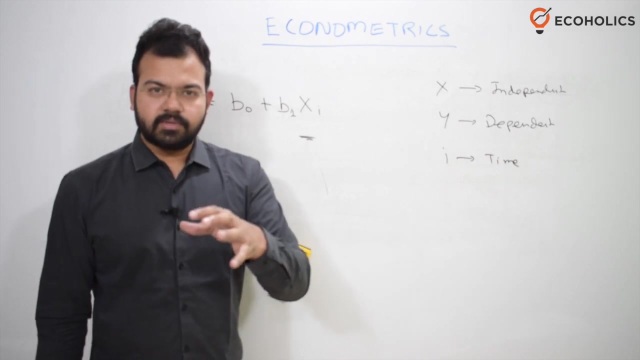 data, cross-sectional data, panel data, etc. So here this Yi small, i refers to certain time period. Now, what is B0 and B1?? Here B0, we can say, is the autonomous consumption, Like, for example, if you are not having any income, but still you are consuming something. 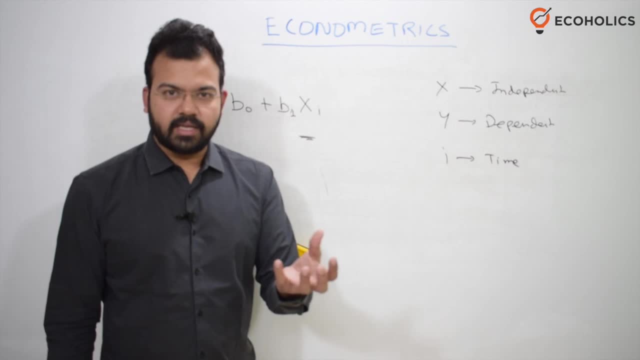 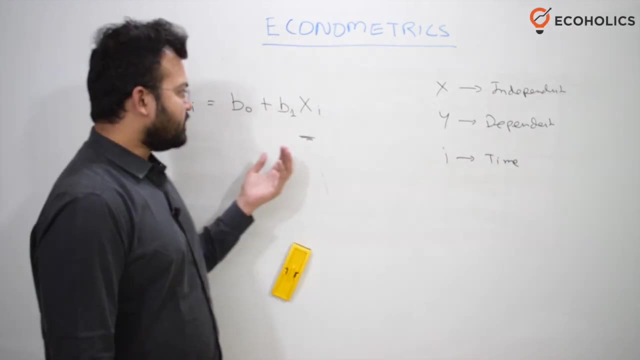 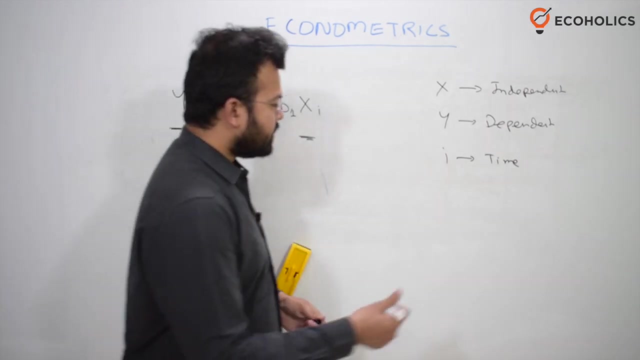 like by dis-saving, like by borrowing money, by begging. So this B0 refers that there must be some autonomous consumption that is affecting the particular consumption. Now here we can say B1,, B1 is the proportion. So in the consumption function we have one. 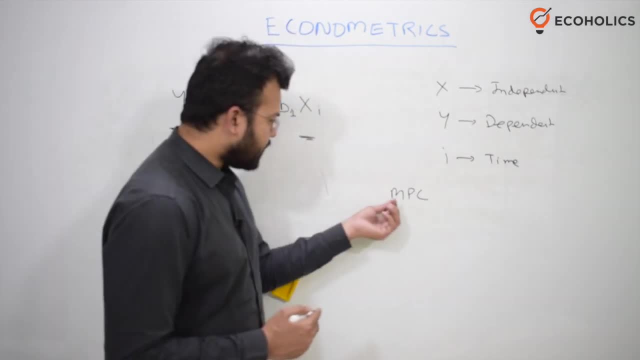 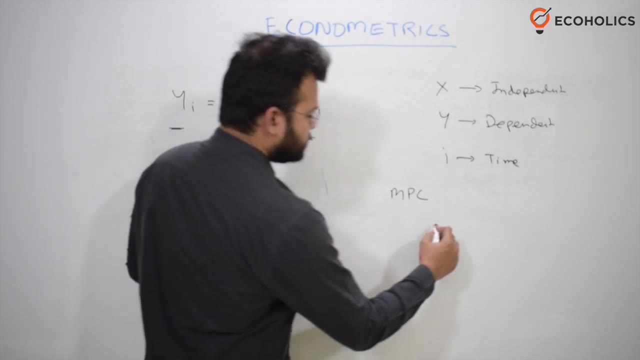 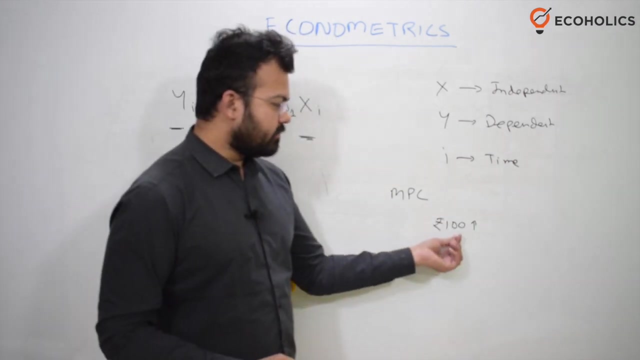 variable that is known as MPC. that is, marginal propensity to consume. It means how much extra income you will consume. Like, for example, you will experience Rs 100 incremental in your particular income. Suppose in a monthly income you will get Rs 100 extra. So from 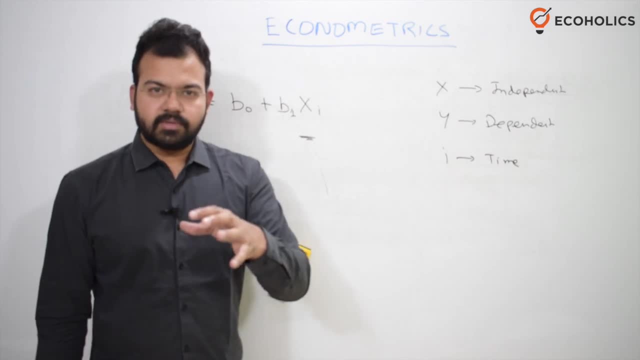 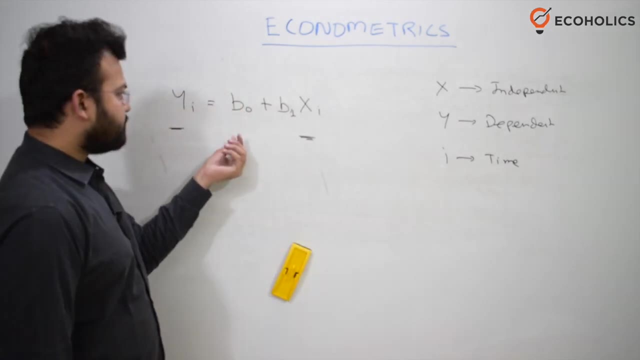 Like, for example, if you are not having any income but still you are consuming something like by dis-saving, like by borrowing money, by begging. So this B0 refers that there must be some autonomous consumption that is affecting the particular dependent variable. Now here we can say B1, B1 is the proportion. 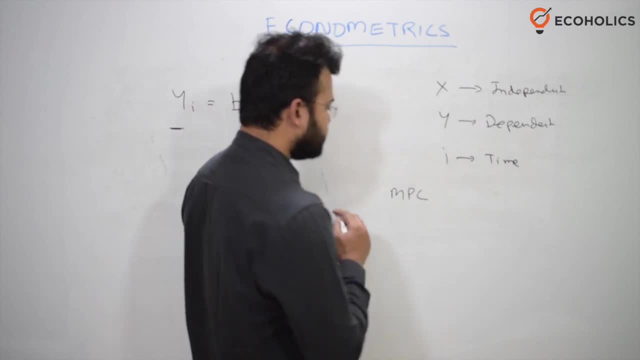 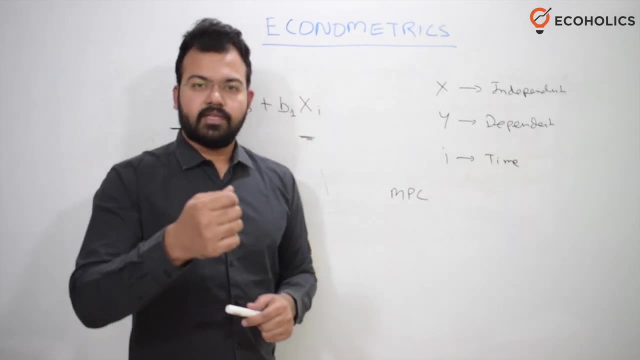 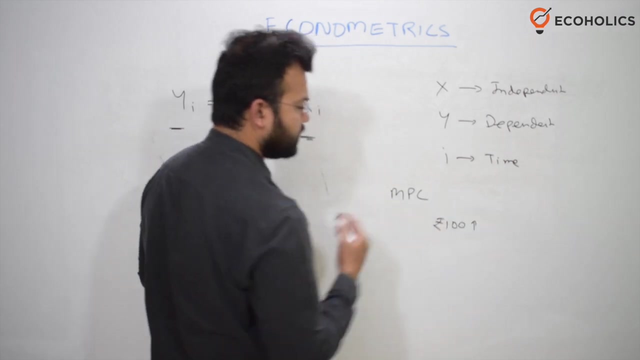 So in the consumption function we have one variable that is known as MPC, That is, marginal propensity to consume. It means how much extra income you will consume. Like, for example, you will experience Rs 100 incremental in your particular income. Suppose in a monthly income you will get Rs 100 extra. 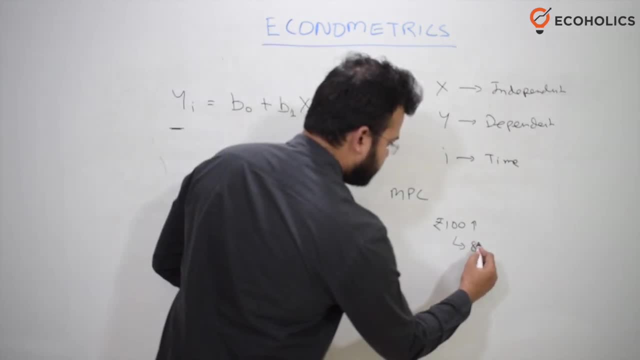 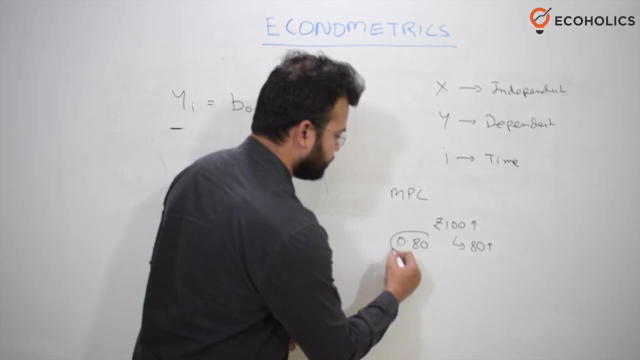 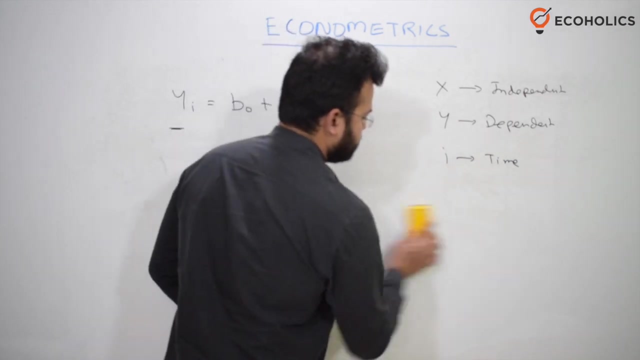 So from that Rs 100. Suppose you will consume Rs 80. It means your marginal propensity to consume is 0.80. So it means with the extra income you are consuming 80% of that extra income, So that B1 represent a certain percentage to that particular independent variable. 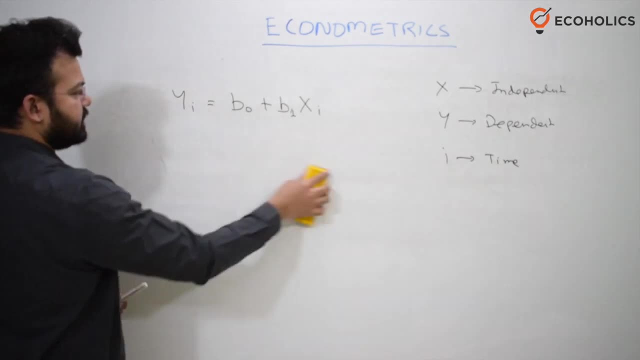 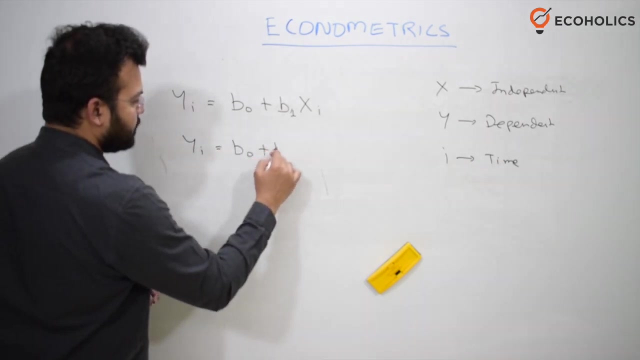 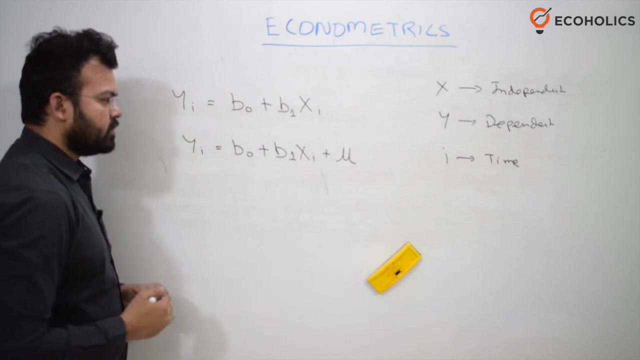 Now in the advanced equation. I have already explained the meaning of this, But you can understand that in the advanced equation, yi is equal to b0 plus b1, xi plus we have to add the mu. This is what we call mu, pronounced as MU. 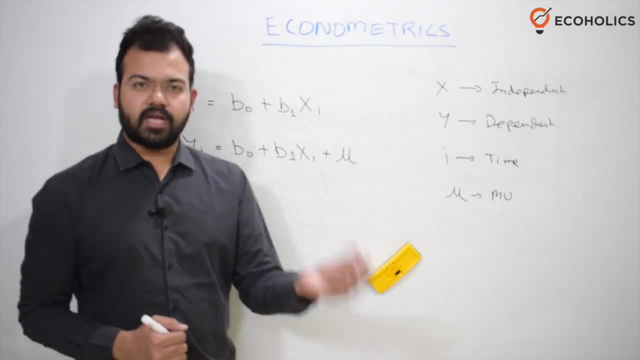 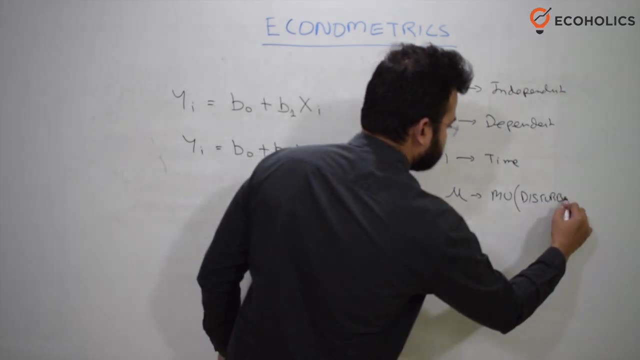 So this is what we call the disturbance term, or the stochastic term or the error term. So this is known as the disturbance disturbance term, We can say the error term or we can say the stochastic term. So these are the terms are very vital. 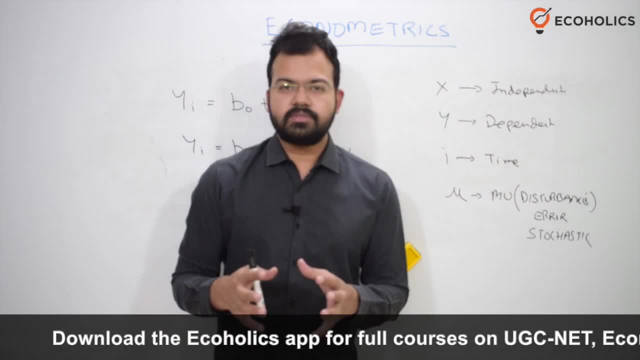 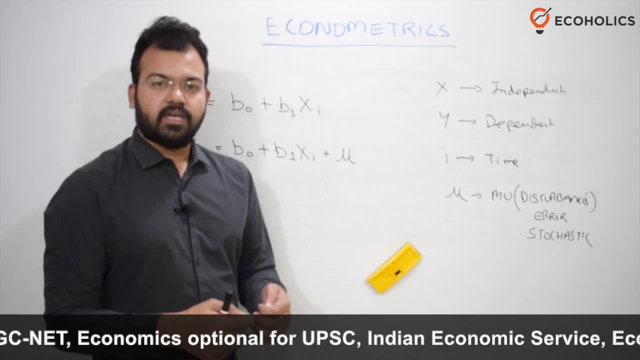 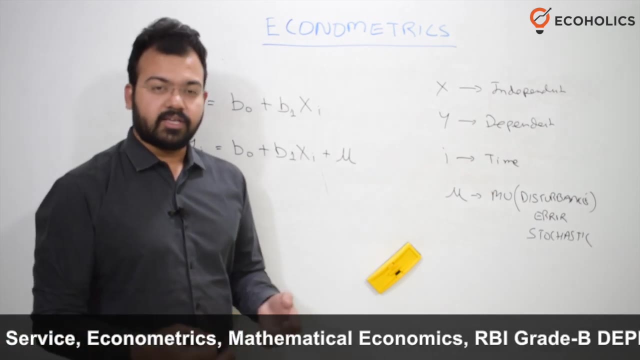 Why? Because, suppose, for example, the consumption is obviously affected by income, But it is also affected by certain tastes, Like, suppose, for example, at night you are, suppose you are having certain idea that we should eat ice cream, But due to the winter season, you are not having that. 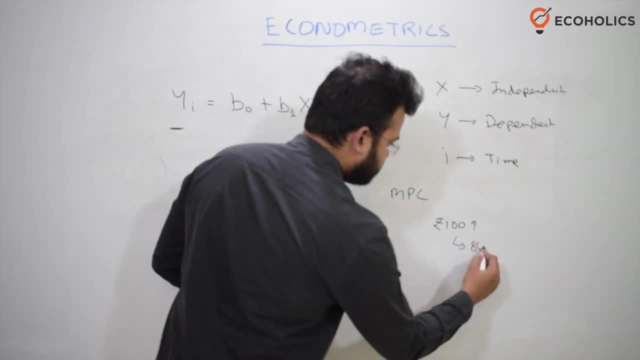 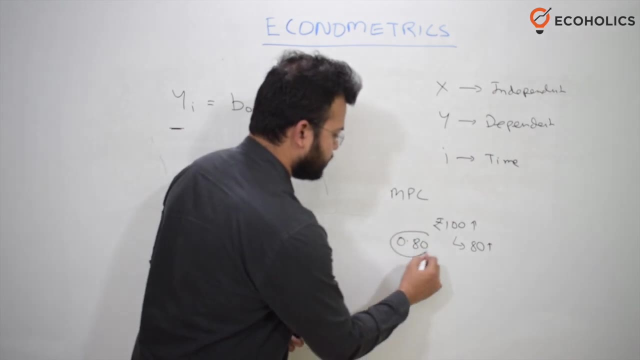 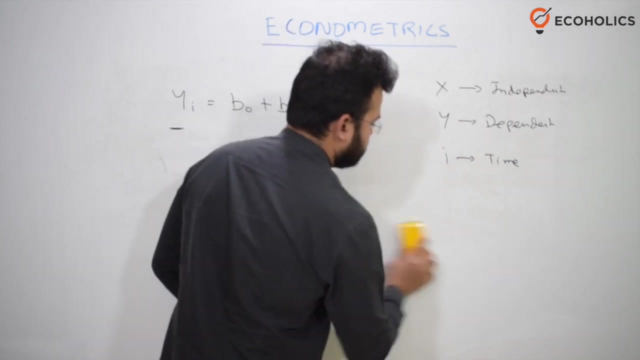 that Rs 100. Suppose you will consume Rs 80. It means your marginal propensity to consume is 0.80.. So it means with the extra income you are consuming 80% of that extra income. So that B1 represent a certain percentage to that particular independent variable. Now in the 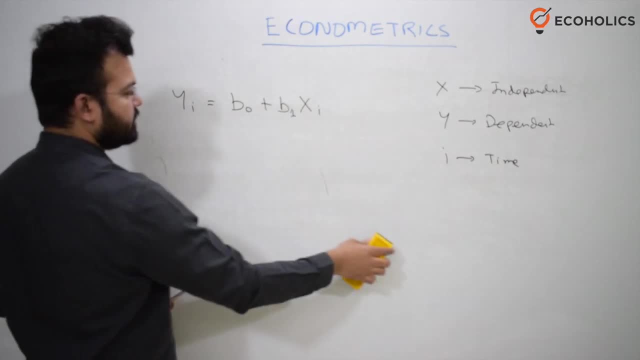 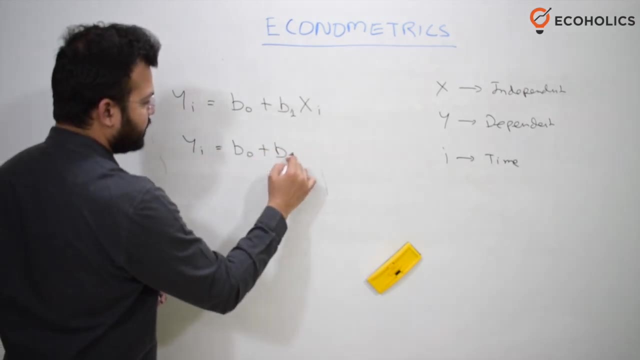 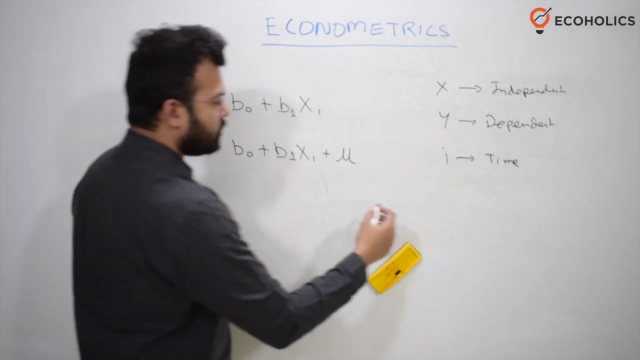 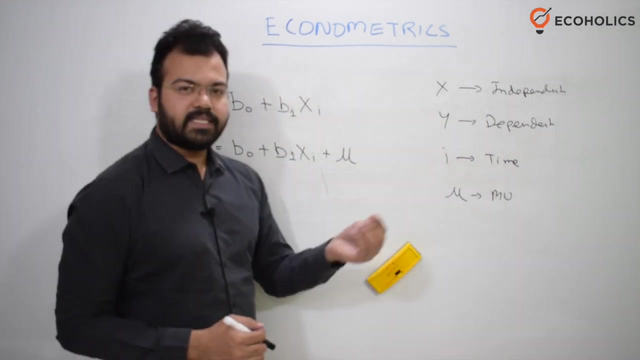 advanced equation. I have already explained the meaning of this, But you can understand that in the advanced equation, yi is equal to b0 plus b1, xi plus we have to add the mu. This is what we call mu, Pronounced as mu. So this is what we call the disturbance term, or the stochastic term, or the error term. 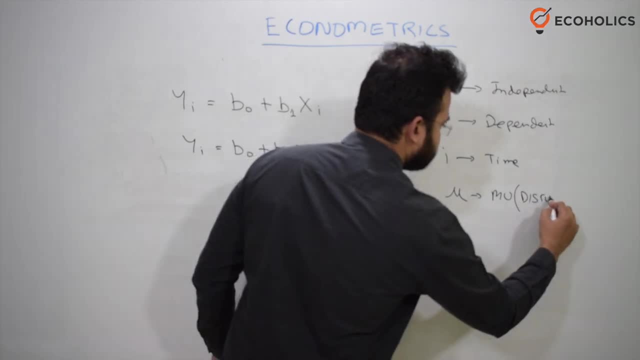 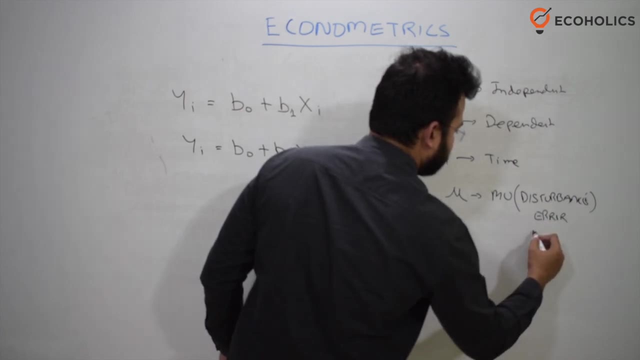 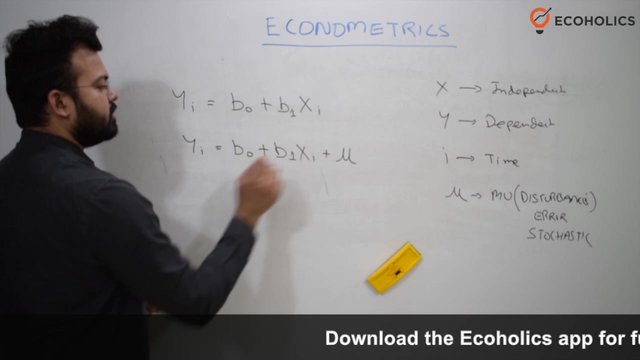 So this is known as the disturbance, Disturbance term, or we can say disturbance term, or we can say the error term, or we can say the stochastic term. So these are the terms are very vital. Why? Because suppose, for example, the consumption. 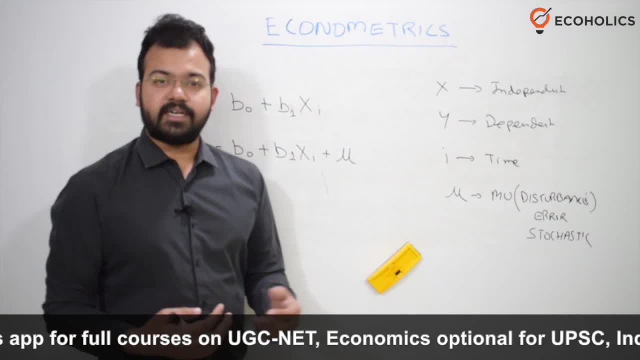 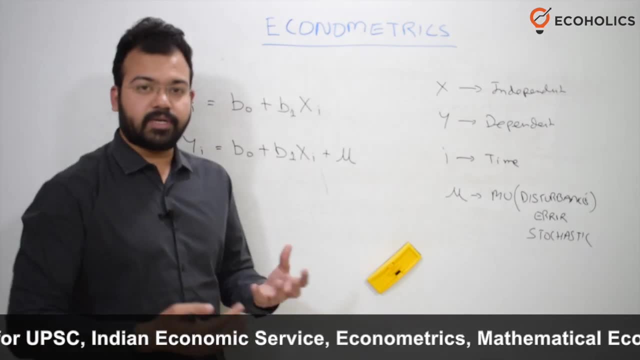 is obviously affected by income, but it is also affected by certain tastes, Like suppose, for example, at night you are, suppose you are having certain idea that we should eat ice cream, but due to the winter season you're not having that. It means weather is considered. 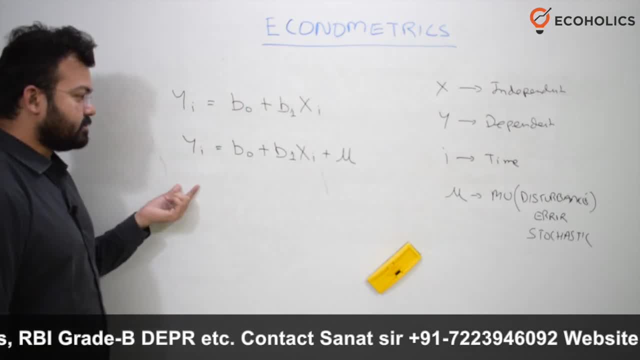 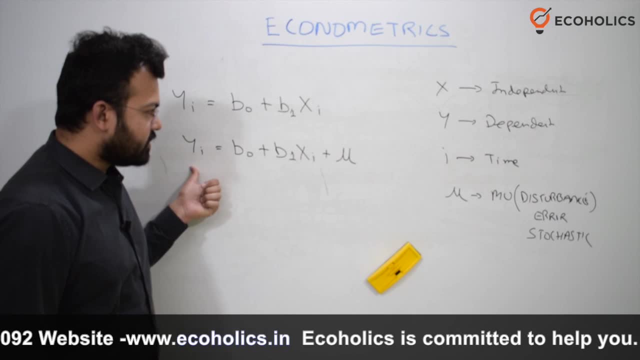 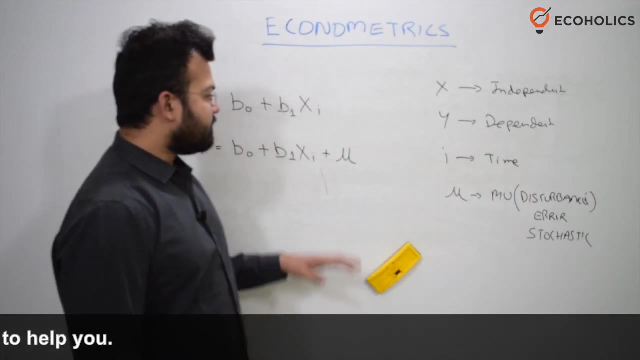 as the external factor that is affecting consumption. But obviously this mu is very small in percentage that is affecting the dependent variable. So that's why we are taking as the error term stochastic or the disturbance term- These are the synonyms you can use. But here we can say this mu is also affecting consumption. 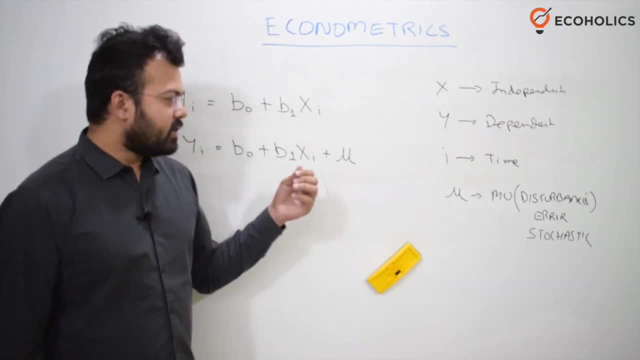 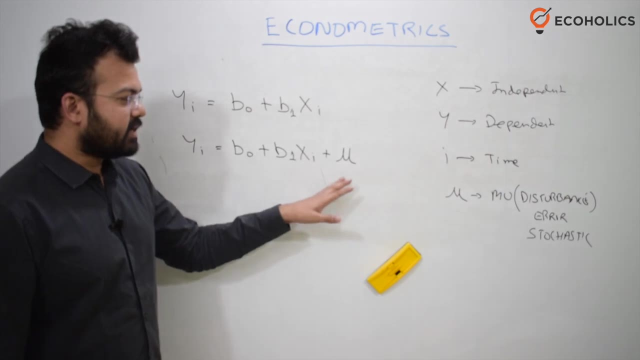 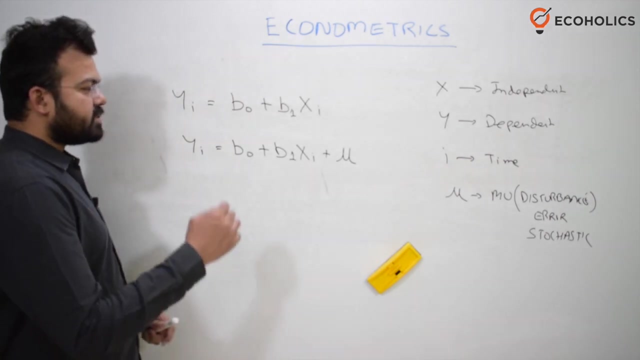 For example, taste and preferences, For example, if your weather is not good, your health is not good- kind of example that we can make for error term. but there are certain kind of assumptions in this econometrics basic equation like, for example, the number one assumption is the mean value of this. 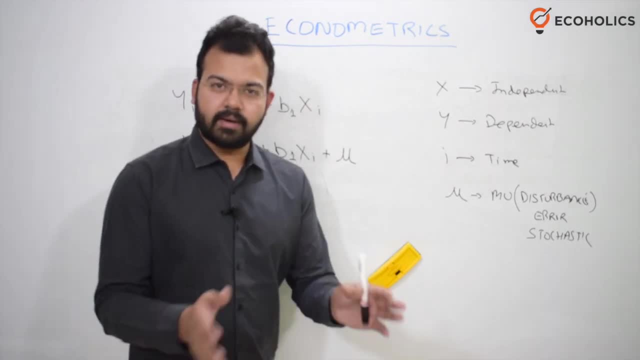 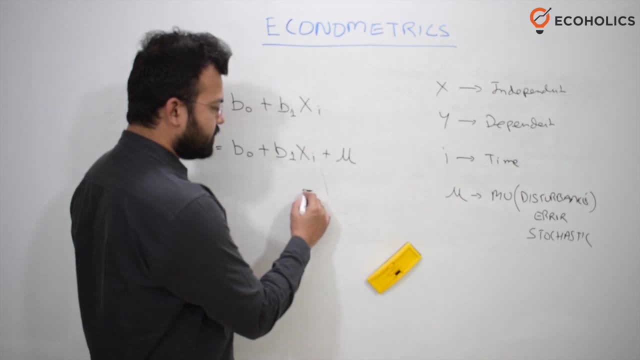 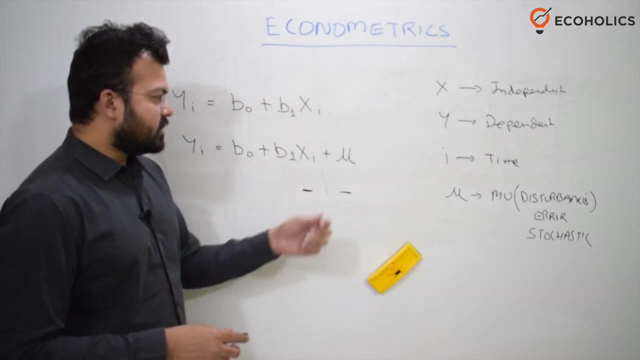 is obviously zero. it means it is not skewed in comparison to the other parts of the variable. if we see this relationship between the independent variable or the error term, so there is no exact relationship that is to be assumed. it means the weather and the income level are not correlated. 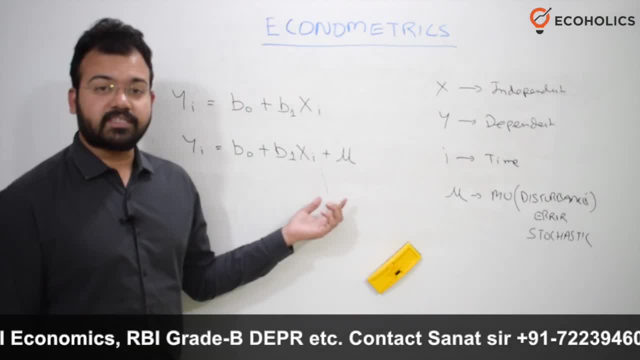 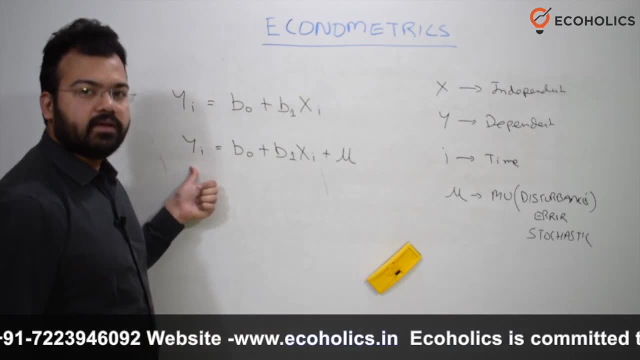 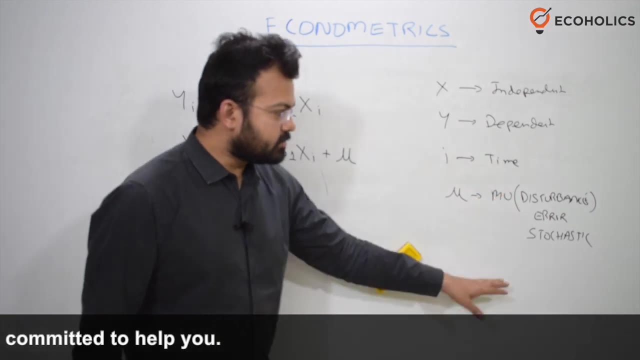 It means weather. So this is considered as the external factor that is affecting consumption. But obviously this mu is very small in percentage that is affecting the dependent variable. So that's why we are taking as the error term stochastic or the disturbance term. These are the synonyms you can use. 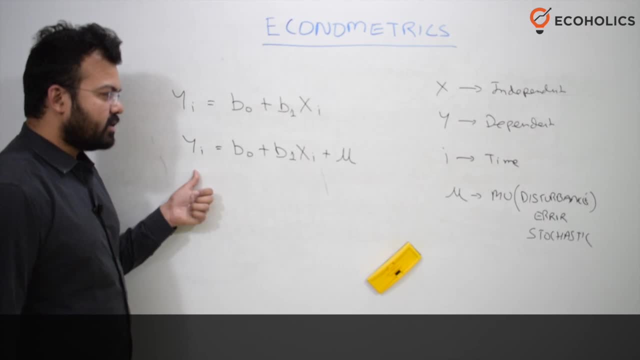 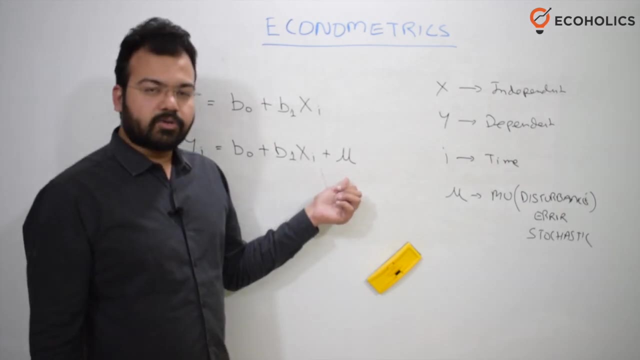 But here we can say this: mu is also affecting consumption, Like, for example, taste, and preferences, Like, for example, if you are suppose your weather is not good, your health is not good. So these are the kind of example that we can make for error term. 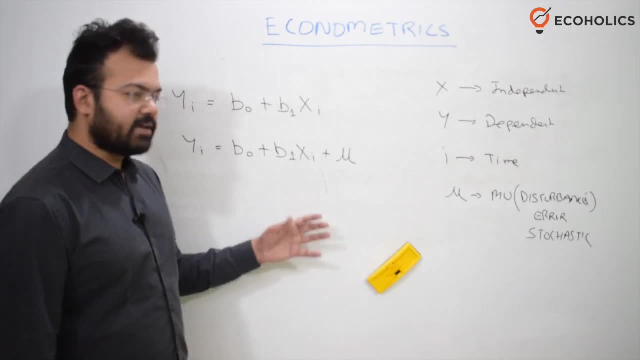 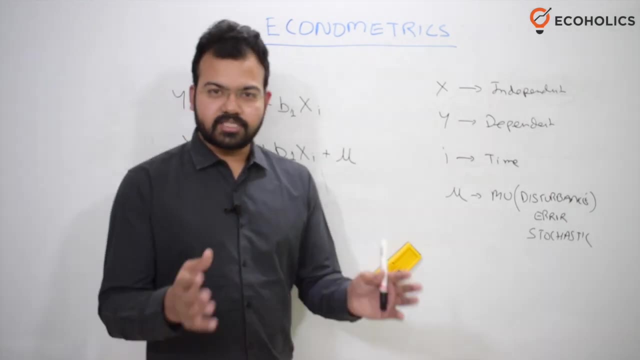 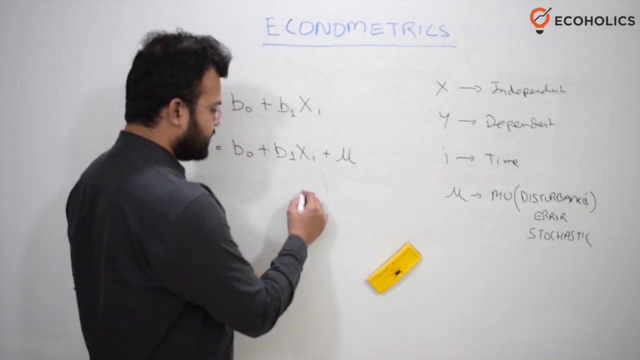 But there are certain kind of assumptions in this econometrics basic equation, Like, for example, the number one assumption is: the mean value of this is obviously zero. It means it is not skewed in comparison to the other parts of the variable. If we see this relationship between the independent variable or the error term, 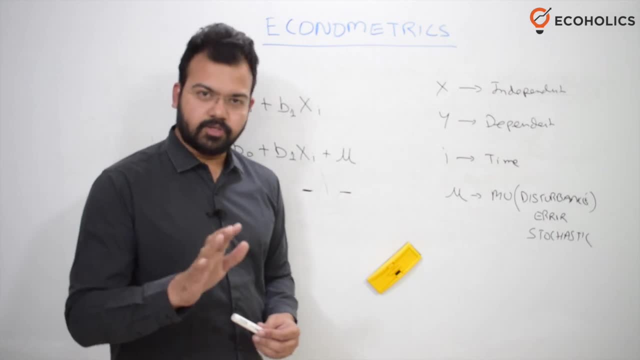 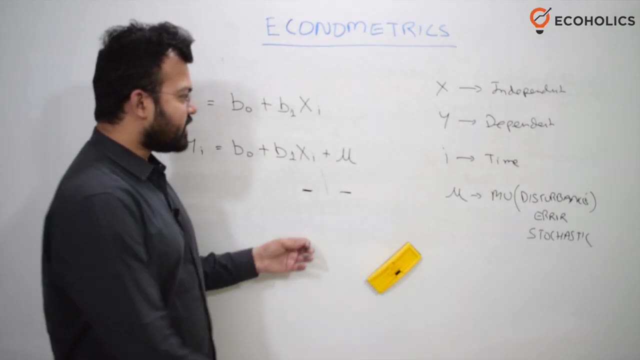 So there is no exact relationship that is to be assumed. It means The weather and the income level are not correlated with each other. So these are the basic assumption that the error term or the disturbance term has to make. So I hope you understand this lecture. 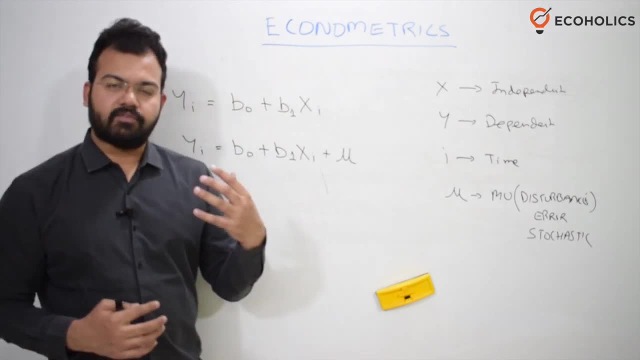 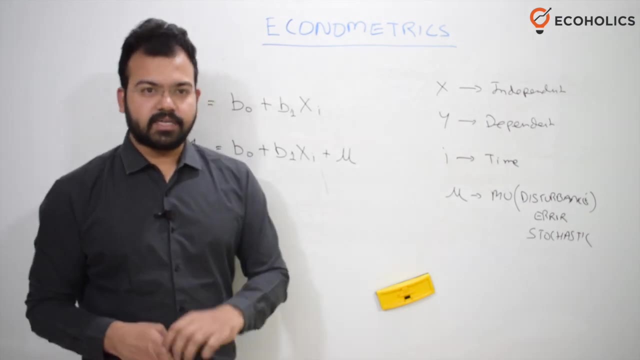 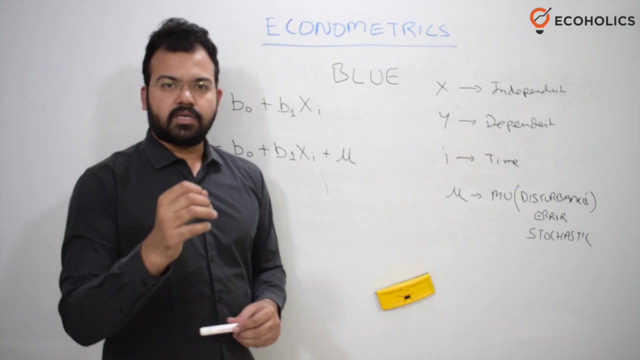 In the next lecture we will discuss certain further advanced equations like ordinary least square method and what is BLUE? that is, best linear unbiased estimator- You must have heard about this term BLUE- and why OLS is considered as the most important, most fundamental method to measure the simple linear regression model. 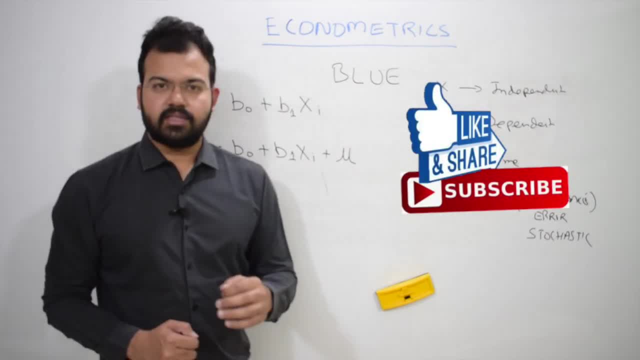 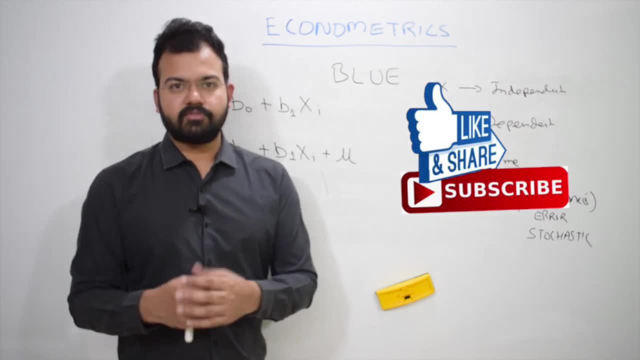 So I hope you understand this lecture. If you have any doubt, you can ask in the comment section, as well as you can ask directly to me on my WhatsApp number. And just if you want more further information, you can visit our website. that is ECOHOLICSIN. 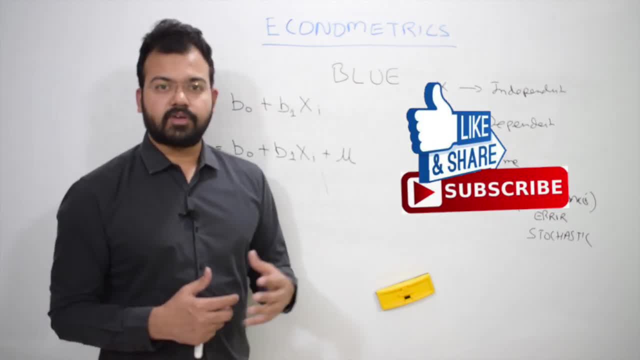 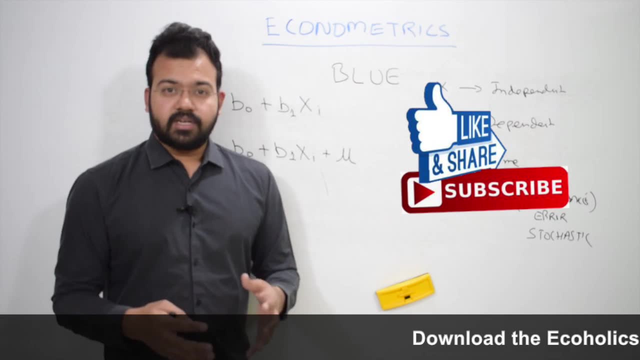 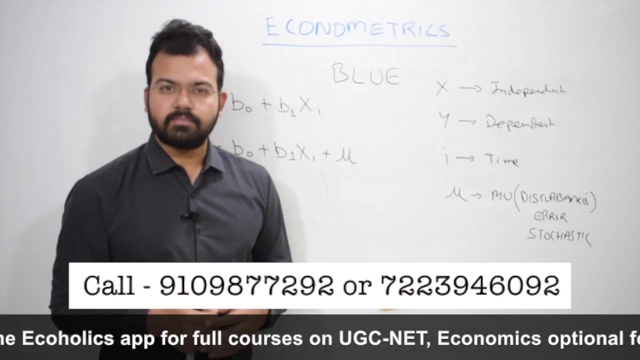 and for more details you can download our app where you have full courses of econometrics, mathematical economics and other major examinations like Indian economic services economics, optional UGC, net, NTA and other basic RBI, grade B, etc. examination. So for more details you can call on these number. you can visit our website or you can. 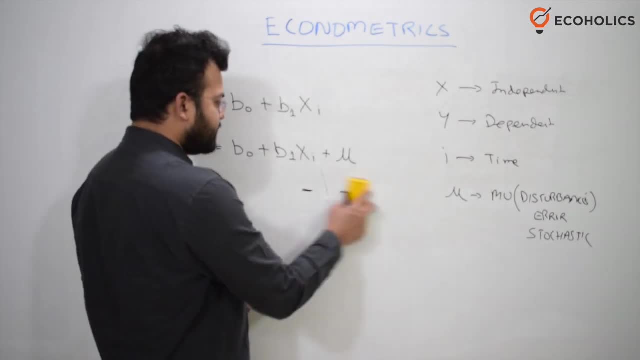 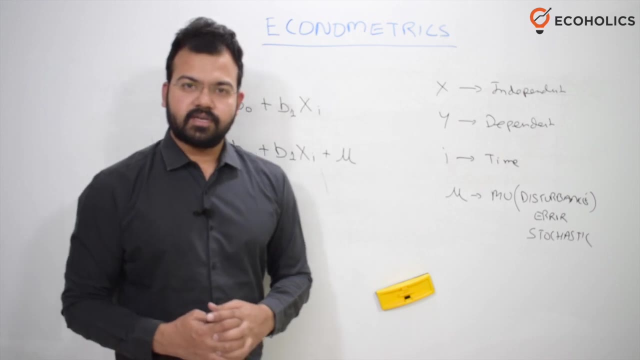 with each other. so these are the basic assumption that the error term or the disturbance term has to make. so i hope you understand this lecture. in the next lecture we will discuss certain further, further advanced equations, like ordinary least square method and what is blue that is best. 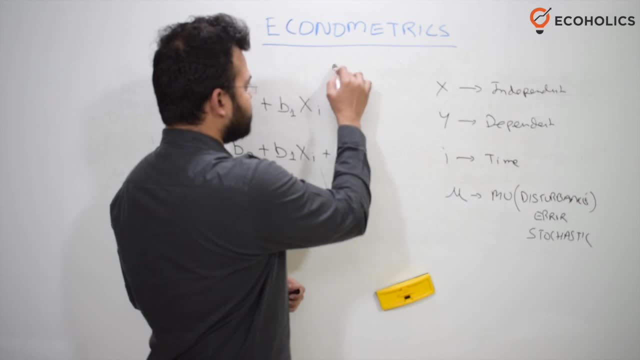 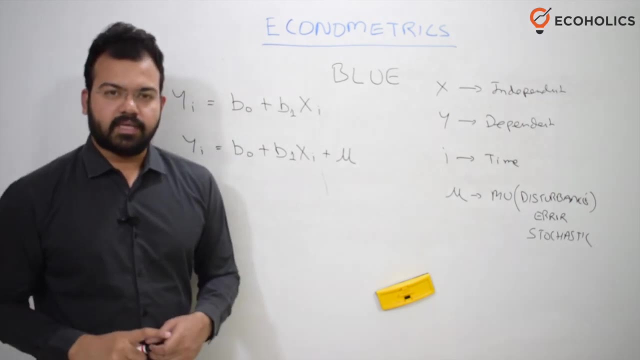 linear unbiased estimator. so you must have heard about this term b l u e and why o l u e is not correlated with each other. so this is the basic assumption that the error term or the as is considered as the most important, most fundamental method to measure the simple linear 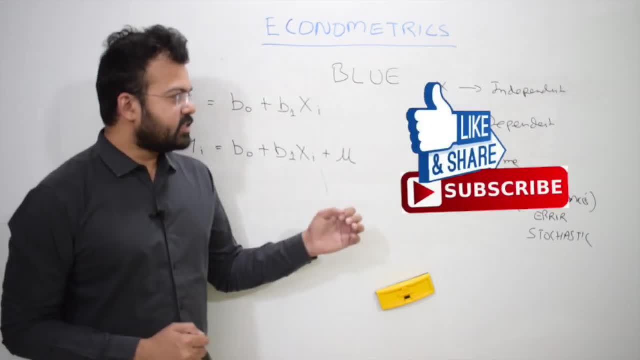 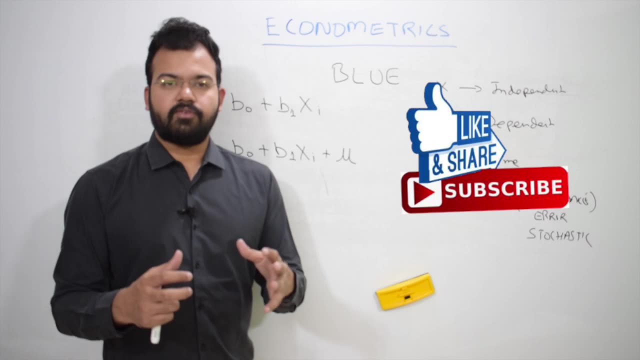 regression model. So I hope you understand this lecture. If you have any doubt, you can ask in the comment section, as well as you can ask directly to me on my WhatsApp number. And just if you want more further information, you can visit our website. that is ecoholicsin. 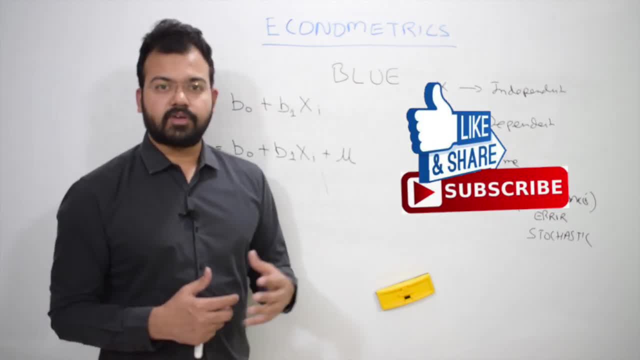 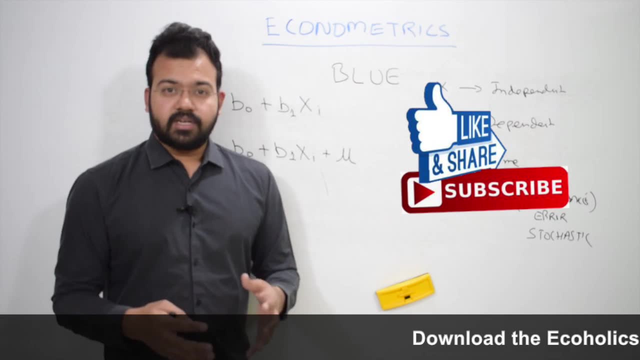 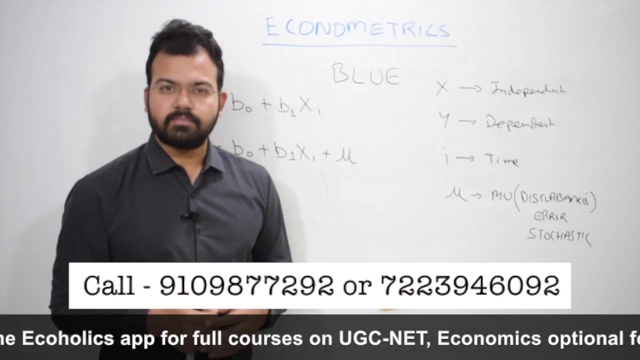 and for more details you can download our app where you have full courses of econometrics, mathematical economics and other major examinations like Indian Economic Services, Economics, Optional UGC, Net, NTA and other basic RBI, Grade B, etc. examination. So for more details you can call on these number. you can visit our website or you can. 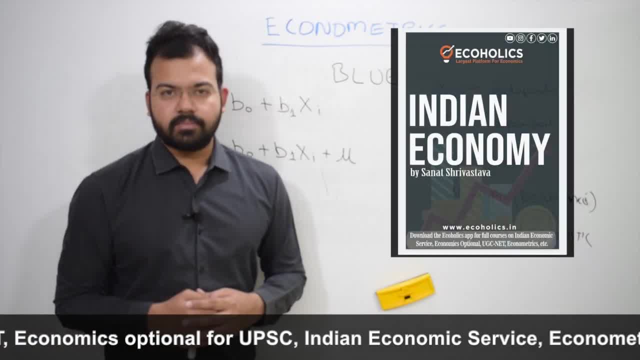 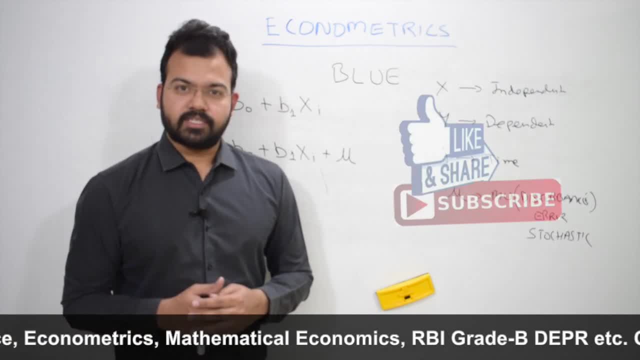 download the app. I have an e-book on Indian economy that is written by me and if you want that free of cost, you can download our app or you can contact on my WhatsApp number. So I hope you understand this And if you like this video. 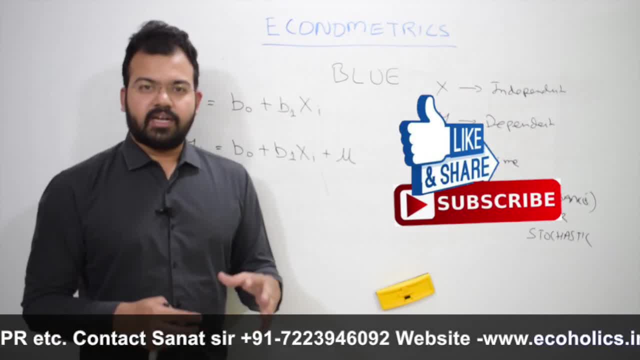 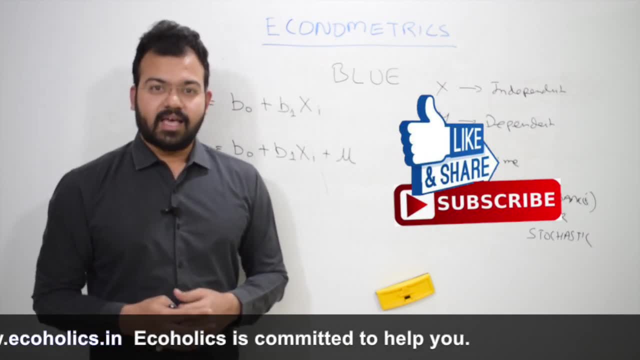 Do comment whatever you want to say about this lecture. It really appreciate our team, that we are working in the right direction And please don't forget to like and subscribe Ecoholics and like this video. if you understand this fully. If you still have any doubt, you can always ask. 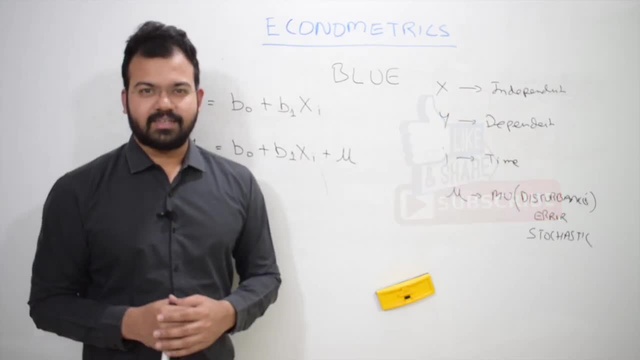 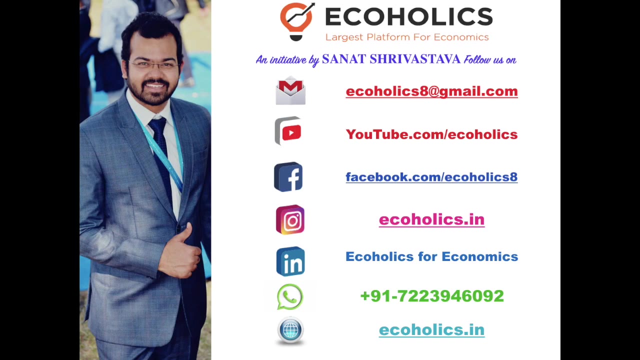 Most welcome with your doubts. So till then, see you soon and have a nice day, Bye, Bye.